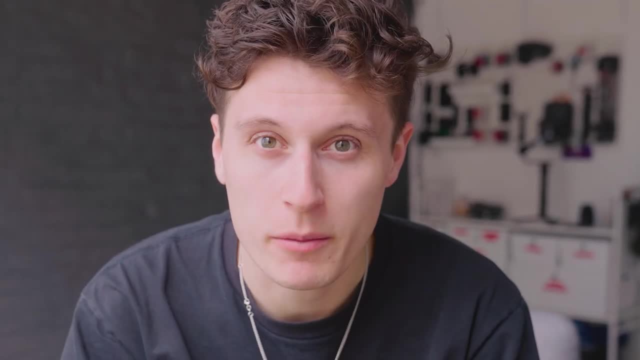 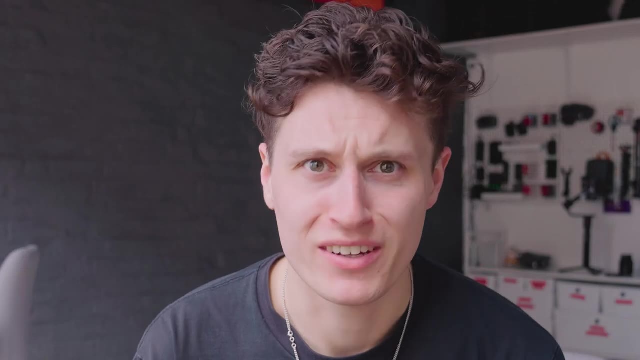 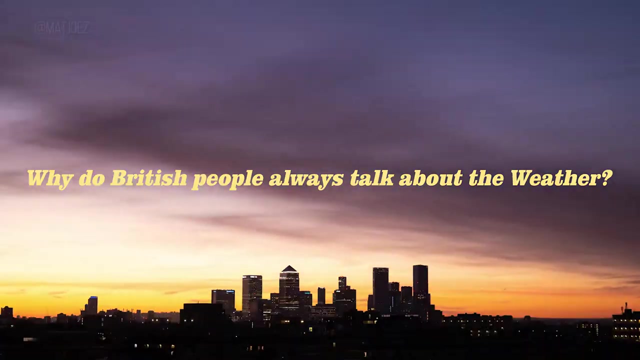 the weather. Get this. we have spent six months of our lives talking about it. No other country talks about it as much as we do, So is it our culture or our climate that makes us so obsessed with talking about the weather? So let's explore that. 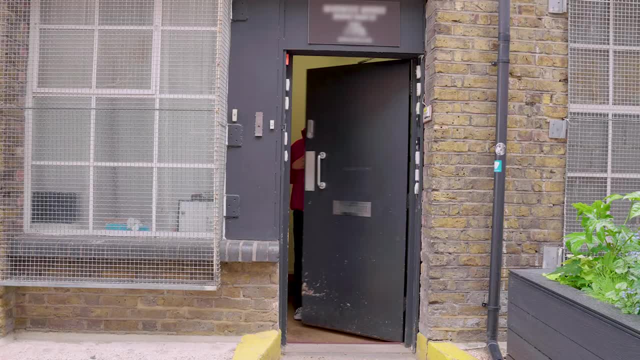 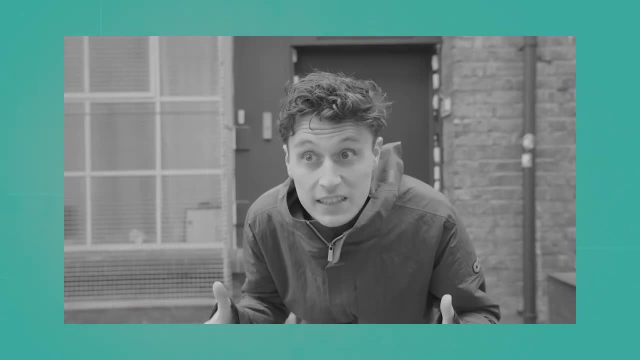 In Britain on any given day. we can be wrapped up against the elements on Saturday, enjoying the sun in a t-shirt on Sunday and battling torrential rain on Monday. I'm waiting all day to shoot the scene and it just won't rain. Maybe that proves my point even more. That's. 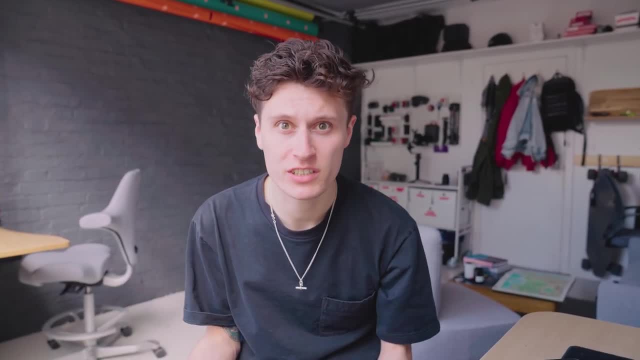 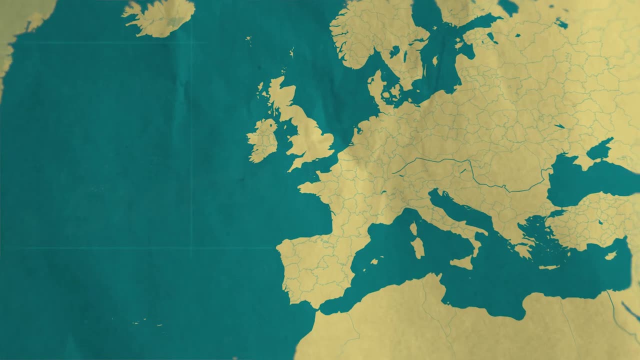 just how it goes. So is there something about the nation's weather that makes it a worthy discussion, or is it just simply a cultural shortcoming that has become a stereotype of Britain? The hell wrote this script. So first let's look at the UK's climate, because there 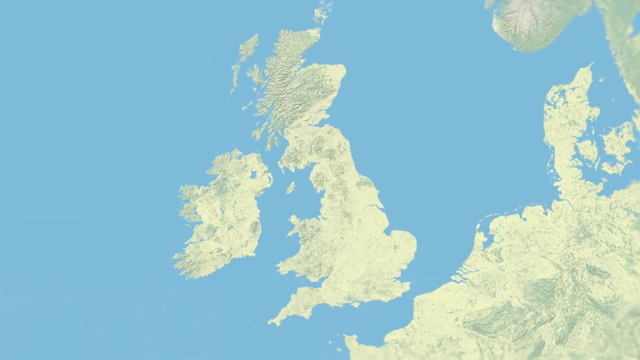 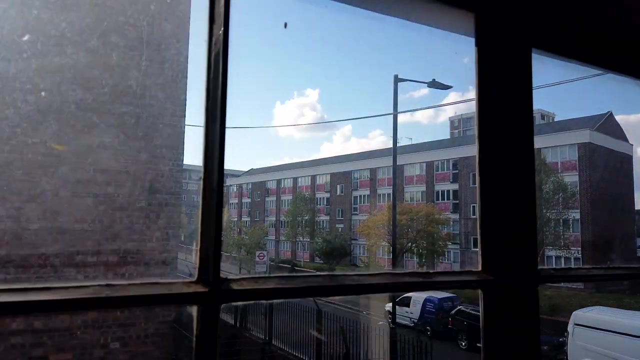 are several features of Britain's geography that makes the weather the way that it is: Mild, changeable and famously unpredictable. The amount I'm having to change the aperture because the clouds coming and going it's just another reason why the weather here is. 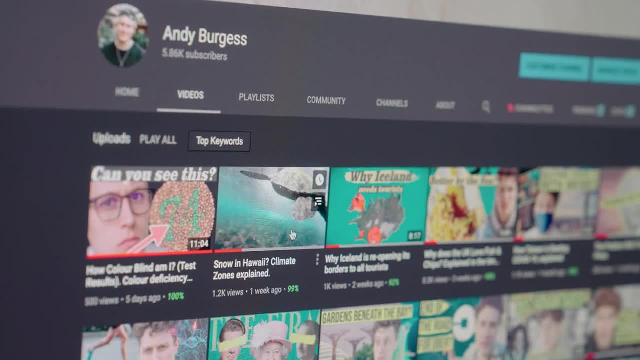 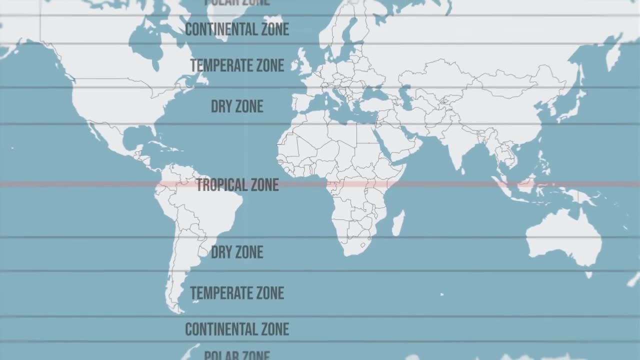 so unpredictable. I released a video two weeks ago on the climate zones of Hawaii and why this one small island in the Pacific has so many different weather types, And in that video we looked at the different climate zones And the UK sits in the temperate zone, meaning 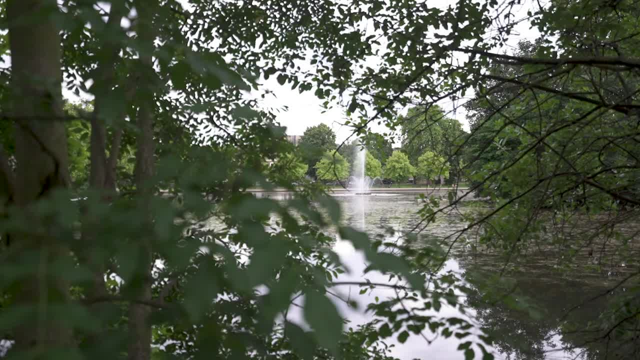 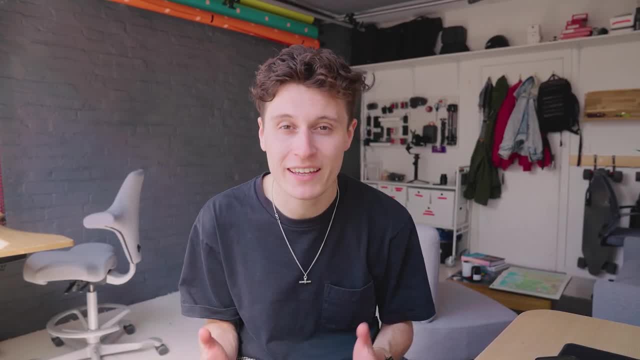 we have all four seasons: moderate rainfall all year round and mild to warm summers and cool to cold winters. The video is linked up here if you want a deeper dive into the crazy climate zones of Hawaii. But back to the UK, Britain's position on the edge of the 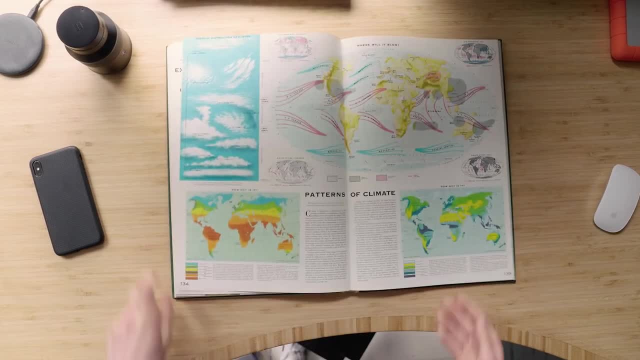 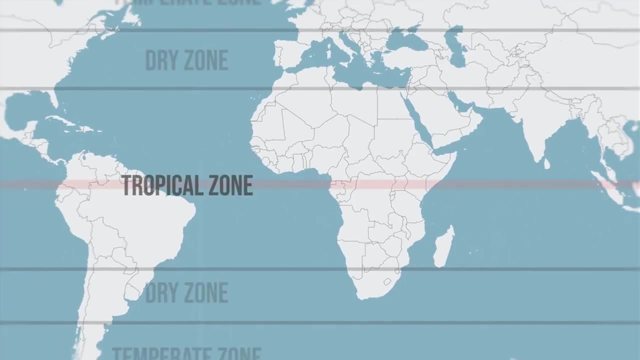 Atlantic places it at the end of a storm track, which are relatively narrow zones of the ocean where storms travel that are driven by prevailing winds, And these storms are feeding on the temperature differences between the equator and the polar zones, As the warm and cold 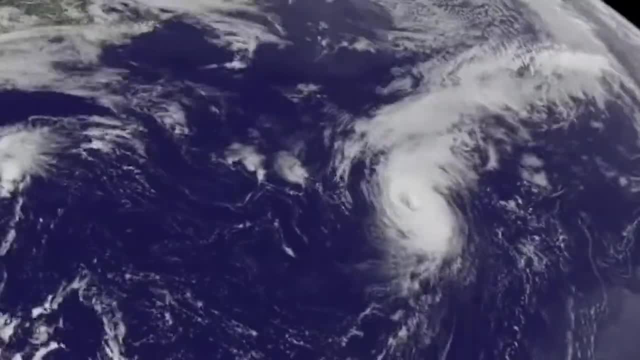 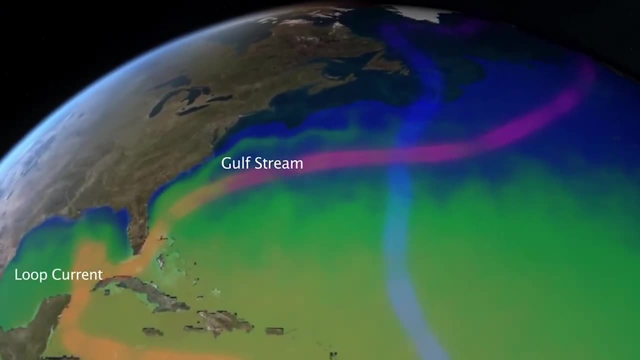 air flow towards and over each other, the Earth's rotations create cyclones, and the UK bears the tail ends of them. You then also have the Gulf Stream, which makes Britain's climate milder than it should be, given its northern latitude And the fact that the UK 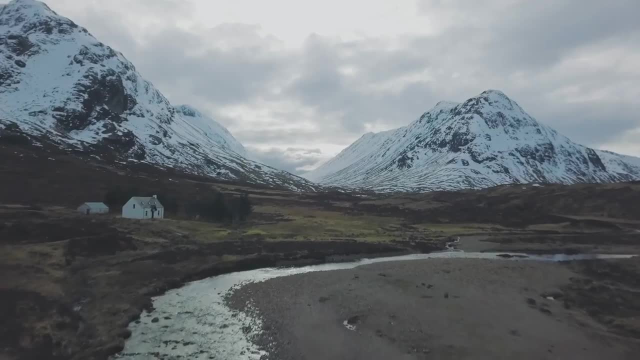 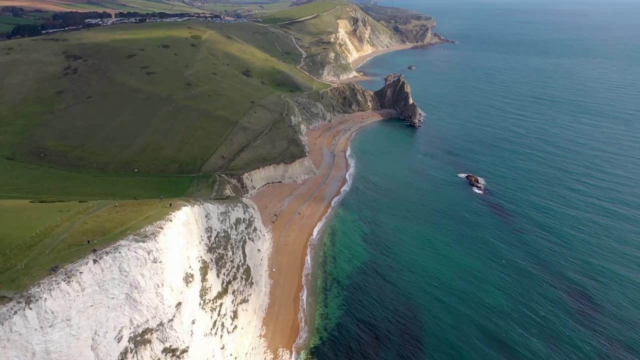 is made up of islands means that there is a lot of moisture in the air and the water in the atmosphere makes the weather particularly unpredictable. Despite our constant complaints, temperatures never really fall below zero and we rarely witness any extreme weather like tornadoes or severe thunderstorms. Yet the lack of consistency means we never quite 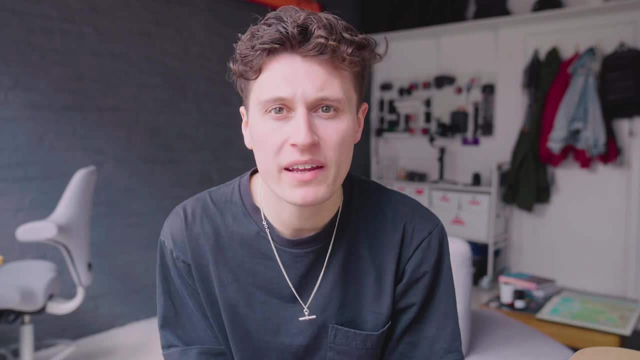 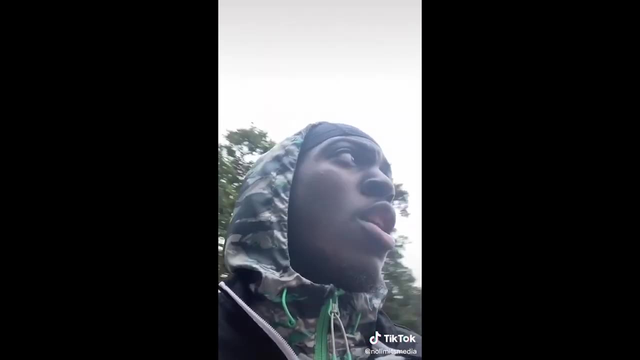 know what to expect day to day. It's a much more unpredictable climate than many other countries. Fam: one second is raining, next second is sunny, next second is hail, next second is earthquake. In fact, there's no volcanoes in England, but I'm sure we'll have a volcanic. 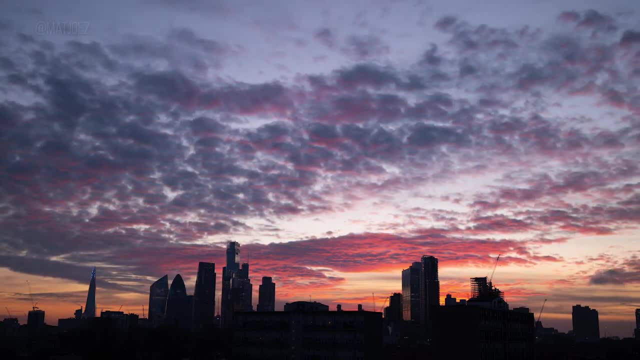 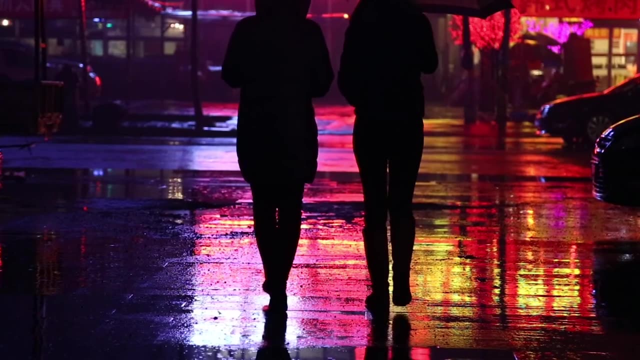 eruption in five minutes. So it's these types of extreme fluctuations that make it such a hot topic in British conversations. So now let's look at the cultural importance of the weather in British society. We just can't cope with snow in this country. Soon as the tiniest snowflake hits the ground. 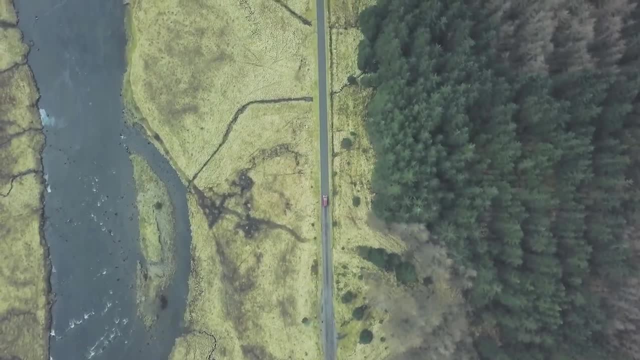 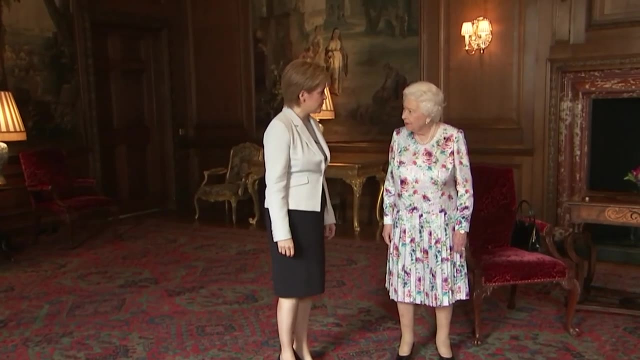 we're like I'm not going out in that blizzard. Most of the day to day conversations that British people make about the weather are pretty mundane and don't really require a response. The weather's been very, very likely. It's gone last afternoon. 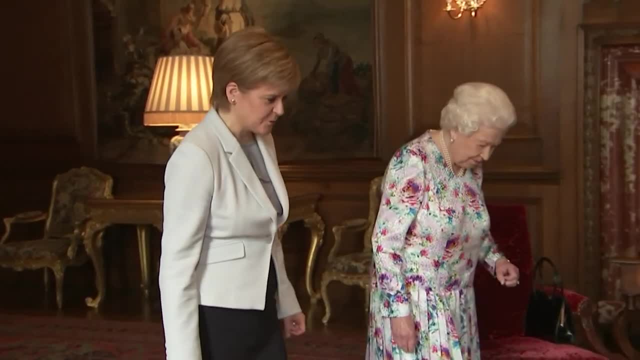 And then, all of a sudden, the sun's gone down, It's gone off, It's gone off, It's gone off, And then all is required is an acknowledgement of that, and then you move on. But it's also a way for us to overcome awkward social situations. 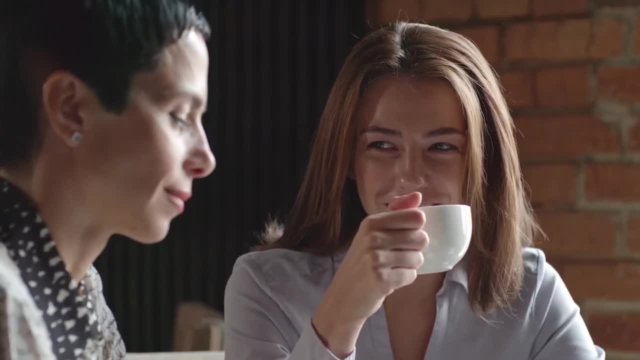 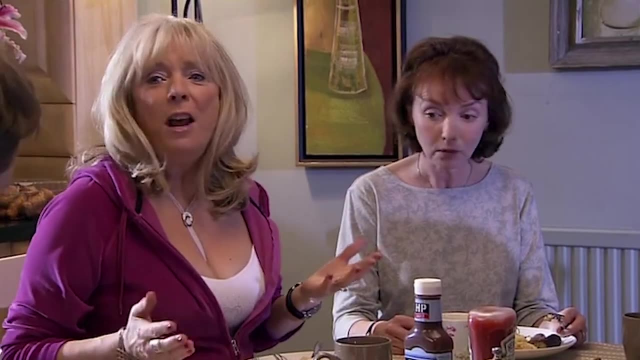 Talking about the weather can be an icebreaker for conversations. It's also used to fill awkward silences or to divert the conversation from an uncomfortable topic. It's going to be a lovely day by all accounts. Yeah, it's going to be nice all week, apparently. 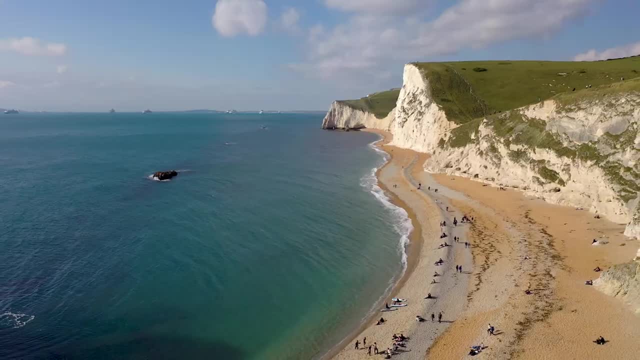 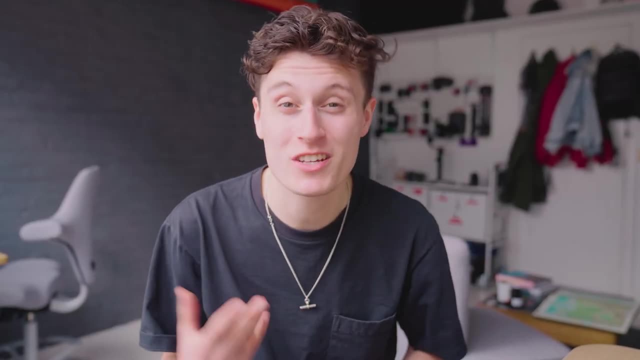 Well, it said in the paper it might rain. Oh really, Yeah, We also use talking about the weather to gauge other people's moods. Depending on the way someone responds to your question about the weather, you can gauge whether they are in the mood to chat or not. 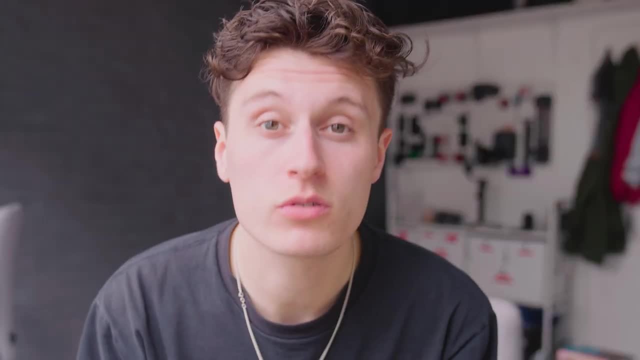 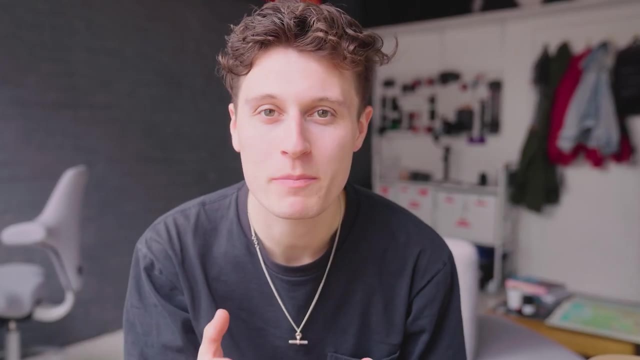 There is also unspoken rules that you must follow when talking about the weather. Firstly, the topic will always be introduced as a question, even if only in intonation, And the response must always be in agreement. It's a lush day, isn't it? 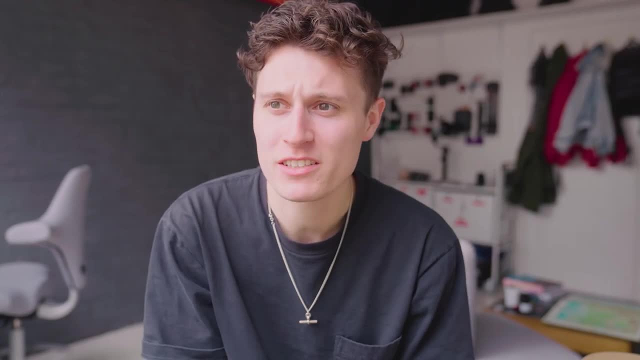 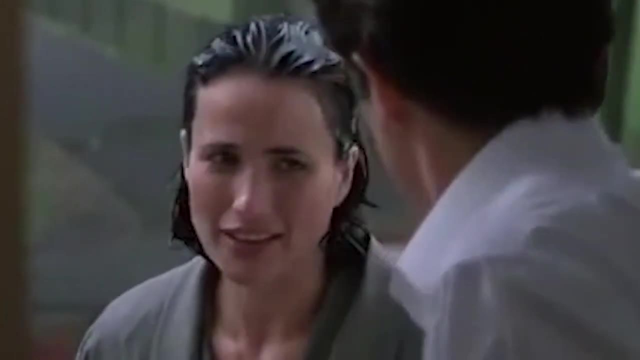 I know we're speaking. If someone disagreed, the other person would be blamed. They would be thrown off guard and really taken aback And feel like this was a discourteous thing to do. And, of course, these kinds of social conversations occur in other cultures. 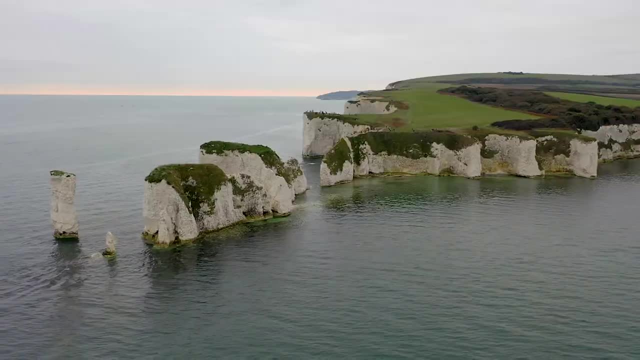 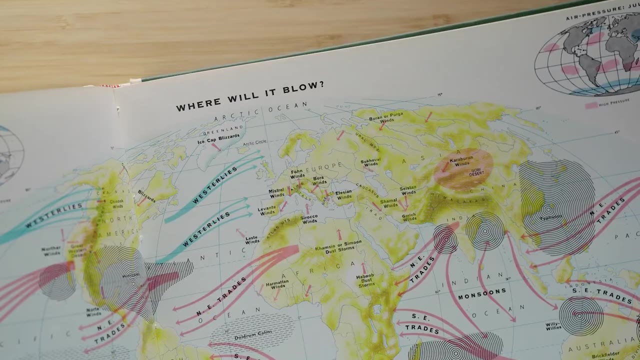 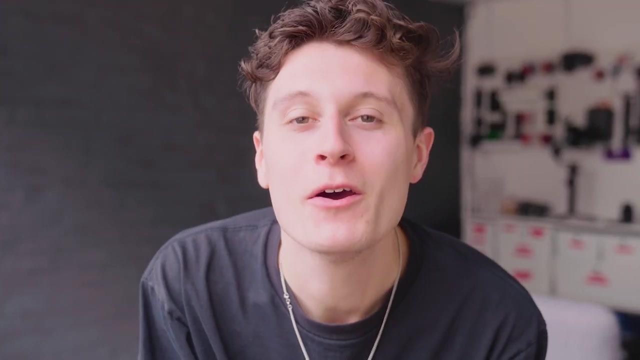 But both the nature of the conversation and their content will vary. I hope you found this short explanation insightful. If you're from the UK, maybe you learned something new about the climate And I'm sure you can relate to having similar conversations. And if you're from anywhere else, I hope this solves the puzzling question of why Brits are obsessed with talking about the weather. 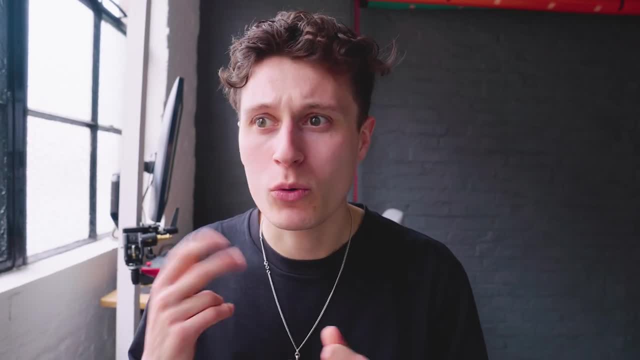 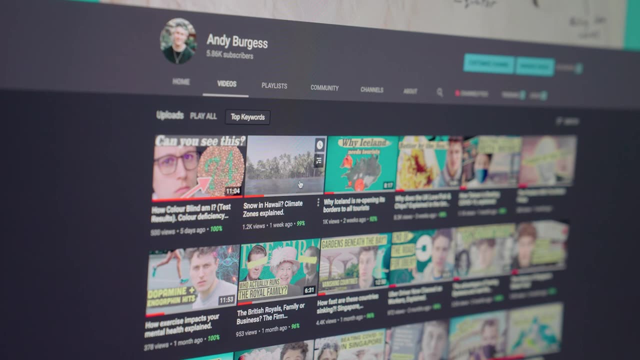 And let me know in the comments below the weirdest conversations that you have ever had with someone about the weather And if you're new around here, my name is Andy. I make word explainers on this channel every Sunday. The goal for this year is to get this channel to 10k subscribers.